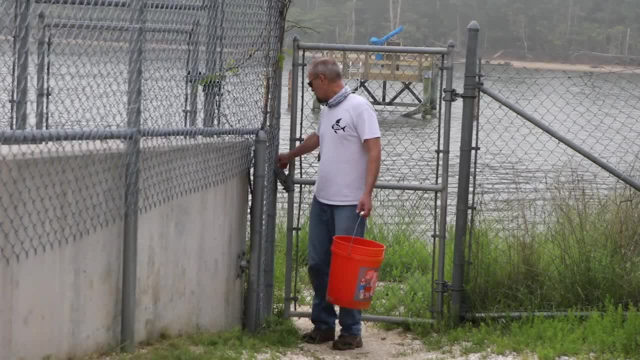 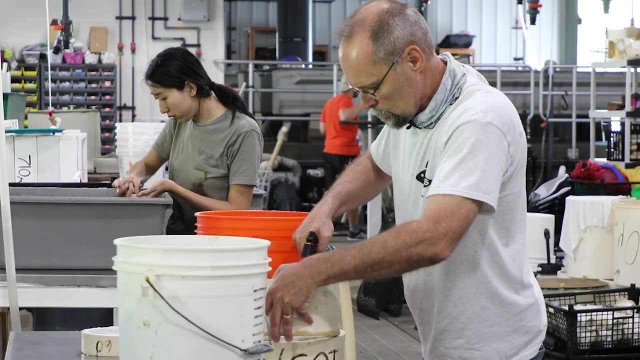 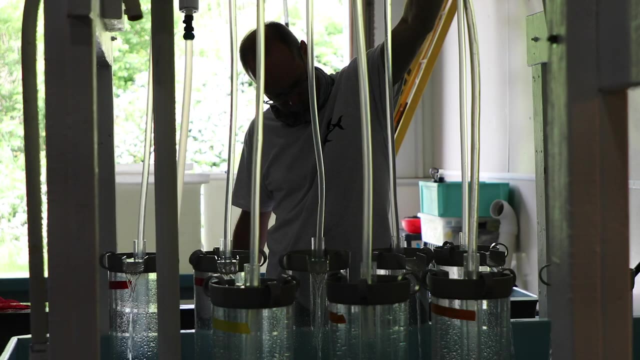 The horseshoe crab head start is a great example of this. The Head Start Enhancement Project at the New Jersey Aquaculture Innovation Center focuses on increasing survival rates of the horseshoe crab's early life history stages along the state's shores. Aquaculture provides a means to give the young horseshoe crabs a jump start. 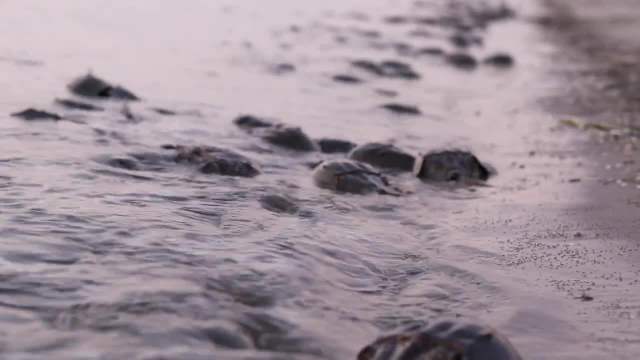 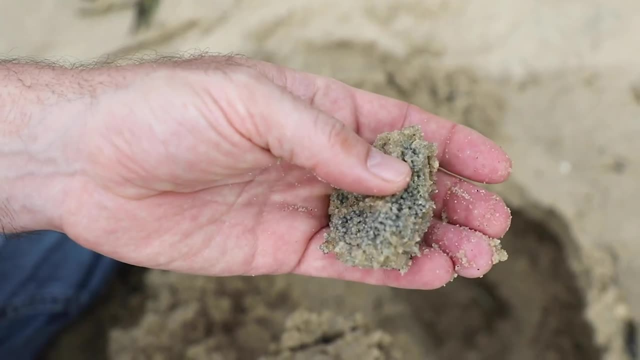 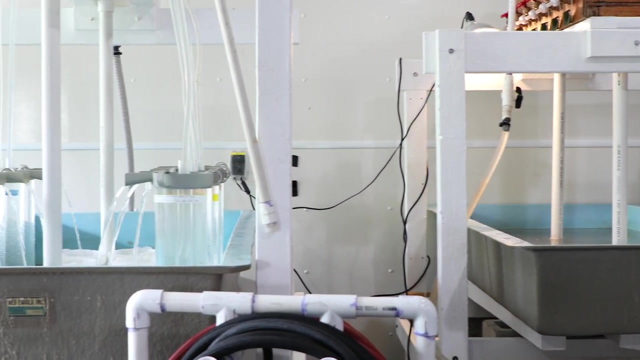 on life. The AIC is piloting research to evaluate the feasibility of large-scale aquaculture of horseshoe crab eggs harvested from suboptimal Delaware Bay birds. An aquaculture setting will provide early life stage horseshoe crabs protection from. 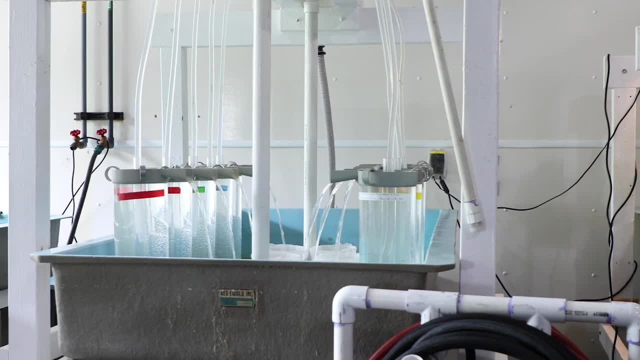 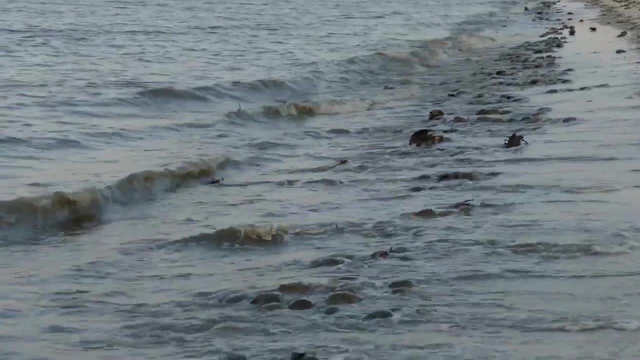 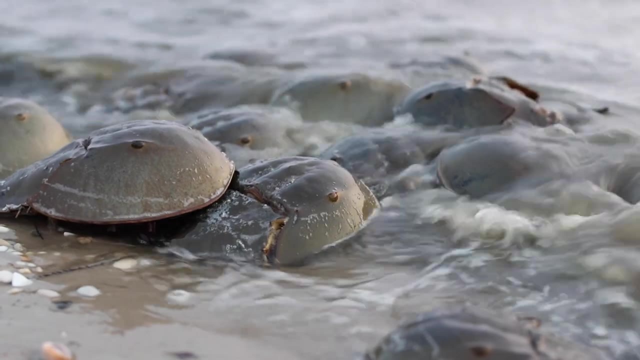 predation and enhance survivorship. Young horseshoe crabs will be released into the wild at four to 12 months of age. Scientists in the region are looking at ways to provide an assurance against further population declines. The Atlantic horseshoe crab is a key species in the estuary's ecosystem because 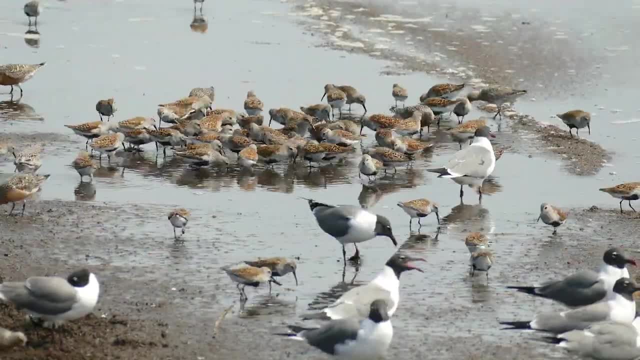 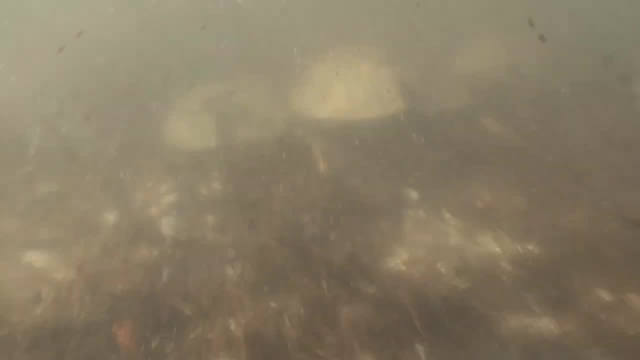 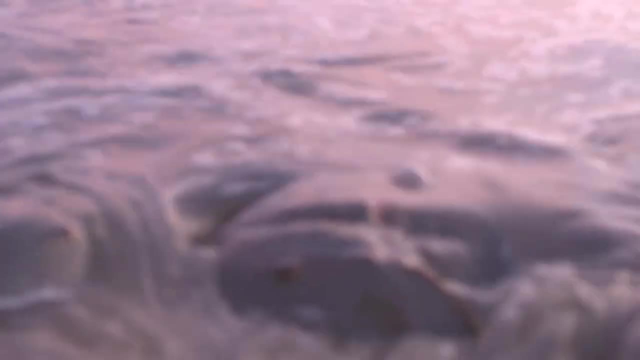 as both food for migrating shorebirds as well as valuable contribution to biomedical research applications. Most of the year, horseshoe crabs reside underwater, but in late April through June, adult horseshoe crabs seek out beaches that are partially protected from surf, within bays and 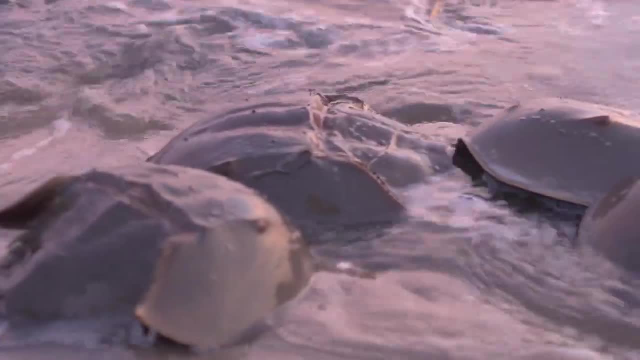 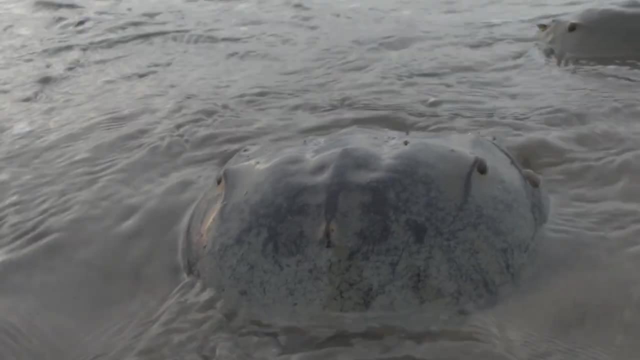 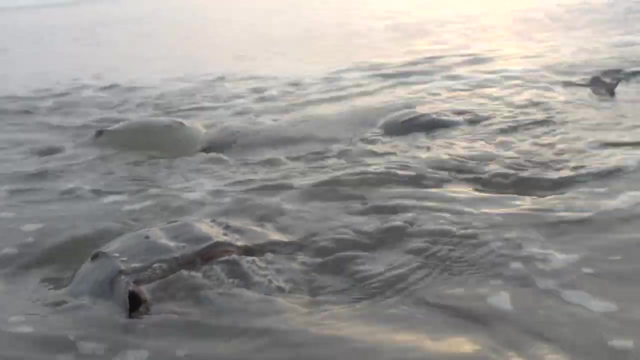 coves to spawn. Peak spawning generally occurs on evening high tides during the new and full moons, As adult female horseshoe crabs emerge from the water, males in tow. they lay eggs in the sand of calm beaches. Female horseshoe crabs generally carry around 80,000 eggs, laying them in four to five clusters of 4,000 eggs each during successive tides. Compared to eggs laid by other animals in the water, these are fairly well protected from predators. In fact, while shorebirds rely on these eggs as creatures, they are also protected from predators. 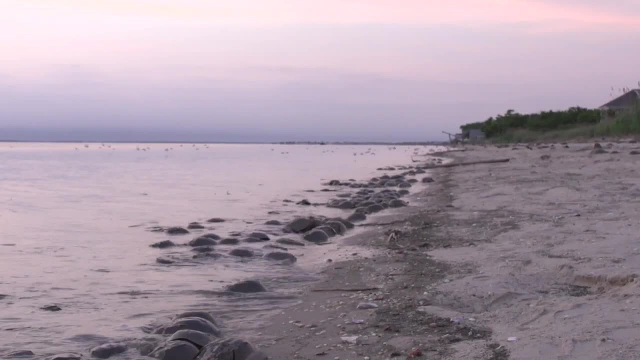 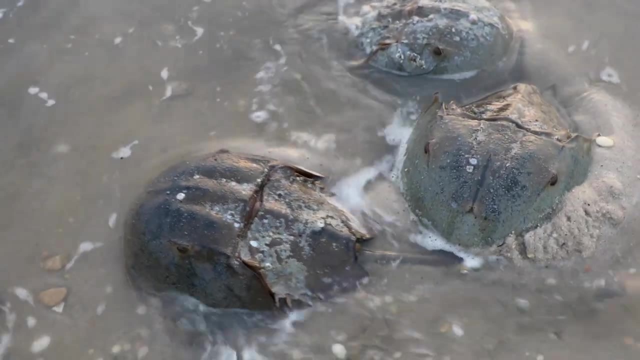 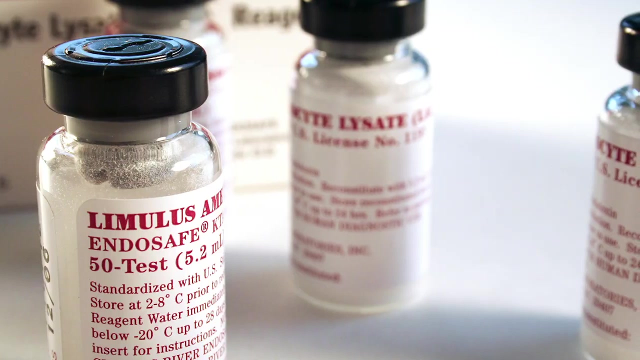 In addition to being a critical fuel for migration, they take mostly eggs near the sand surface that have been displaced from deeper nests by abundant migrating crabs. A decline also has an effect on the human population. The blood of horseshoe crabs contains an important component. 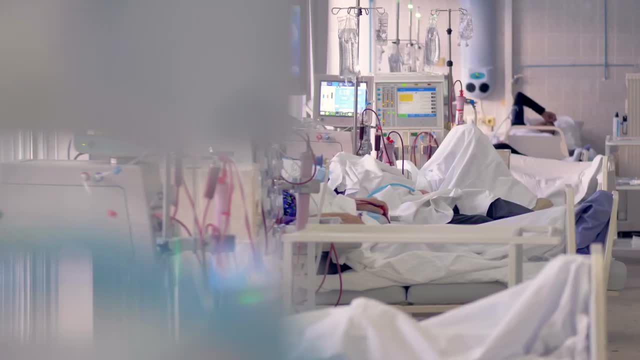 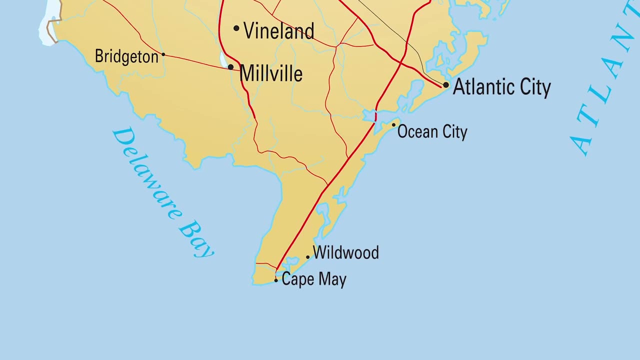 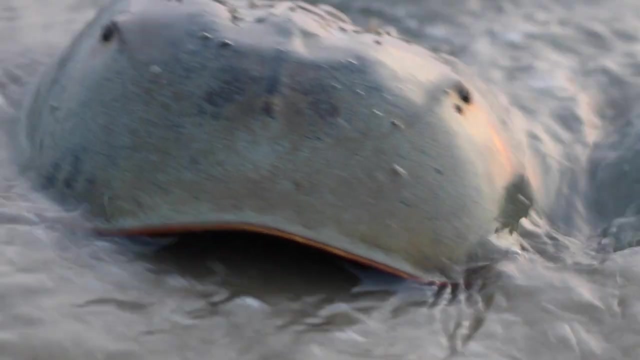 limulus amoebicite lysate, or LAL, that is used to ensure the safety of the world's medicine and surgical supplies. Thousands of nesting female horseshoe crabs will make several trips to lay their eggs. With each trip, the female horseshoe crabs will dig a small nest and lay a series of four to five discrete egg clusters. By the end of the season she will have deposited as many as 20 clusters. By hatching and growing larvae in an aquaculture setting, scientists hope to usher juveniles past this stage to a size where they are more able to fend for. 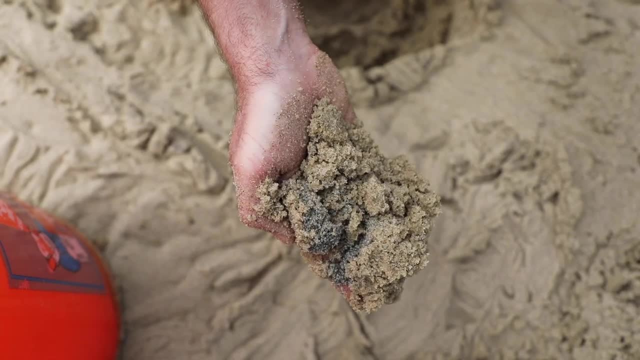 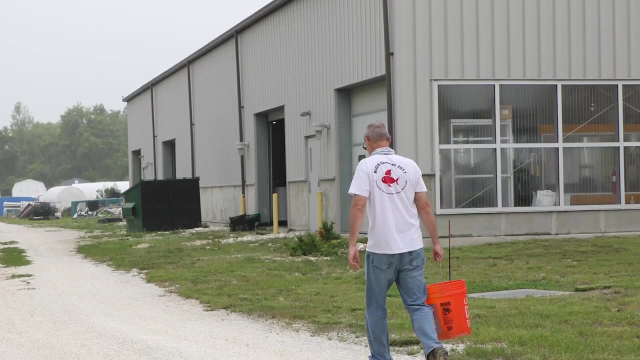 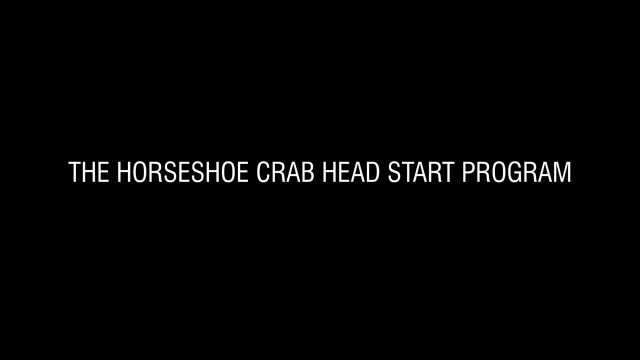 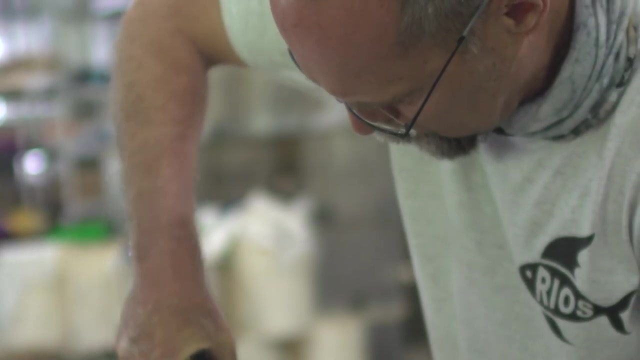 themselves. Using eggs collected from the beach ensures a sample with genes representing local population from individuals that successfully lived in this environment for many years and successfully spawned. The eggs are carefully separated and washed. Some are stored for later use in cool, wet sponges emulating the conditions of the nest. Others are placed 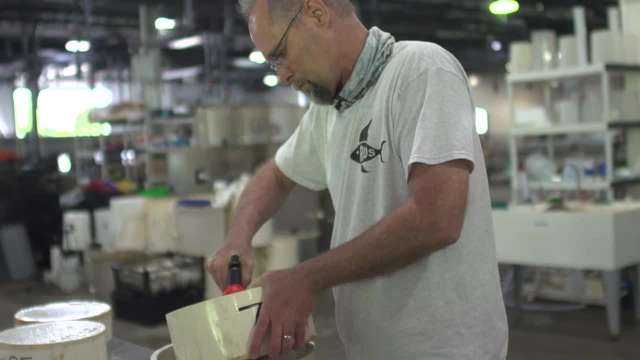 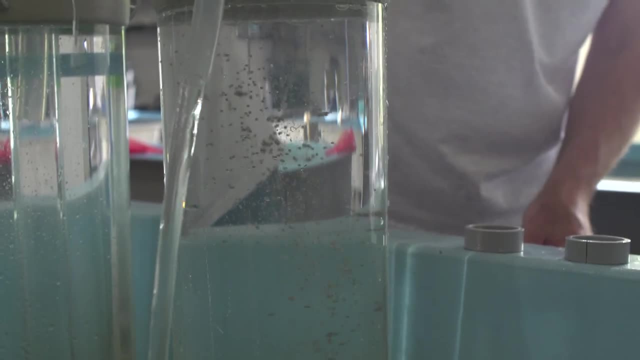 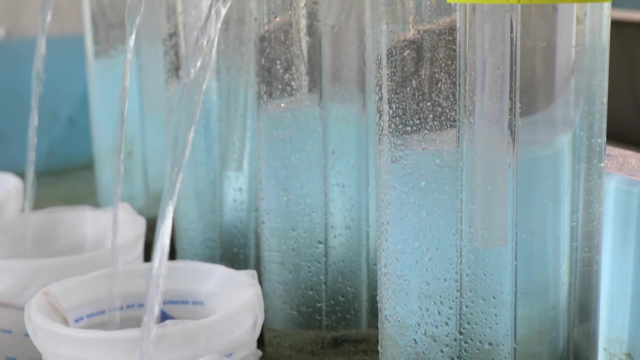 into McDonald jars, Chambers, where they are gently tumbled to make sure they have access to oxygen-rich water and kept free of fungal disease and predation. After several days, the eggs begin to hatch, The larvae struggle free of the shells and begin to swim as they would in the wild When the bubbles in the McDonald jars are. 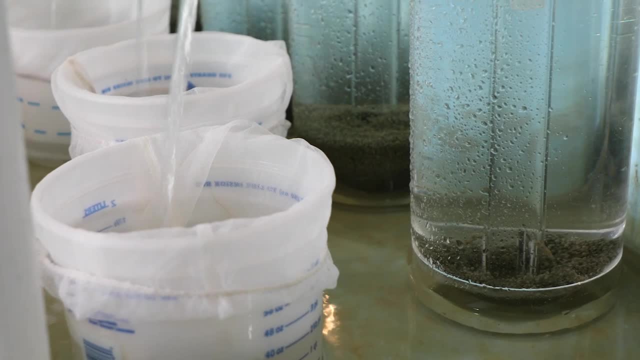 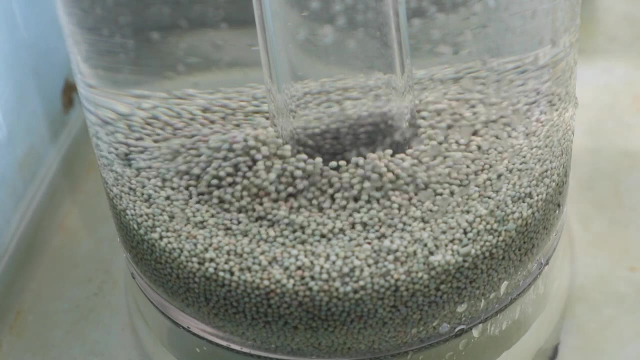 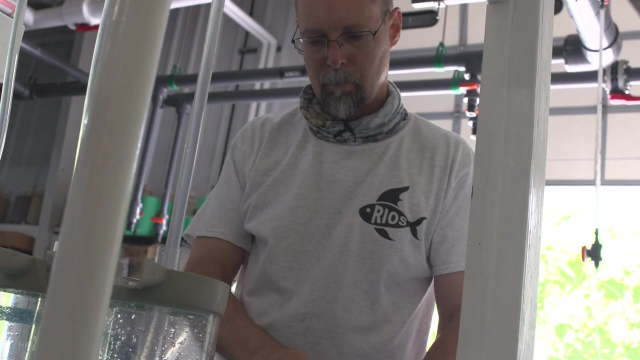 turned off, the empty shells fall into a layer on the bottom and the swimming larvae can be decanted into nursery tanks. At this point, the larvae have used up the energy that they had stored as yolk and need to feed. Because their exoskeletons are hard, they have to regularly shed them and harden. 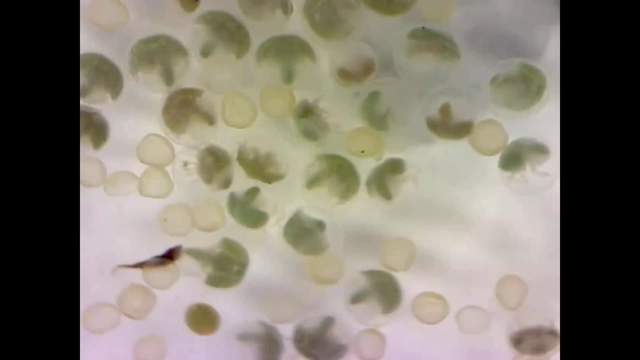 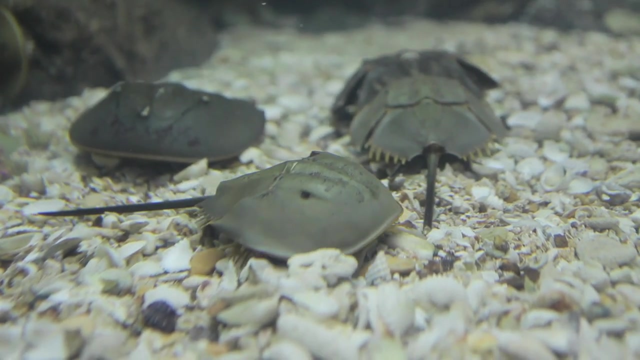 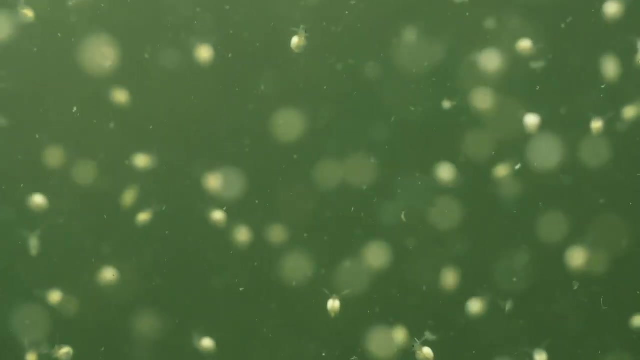 a new layer, into a new shell, in order to grow. Feeding these tiny creatures presents new challenges. They are able to feed themselves from plankton if raw sea water is pumped into the tanks, But this also lets in the eggs and larvae of predators that would eat them. 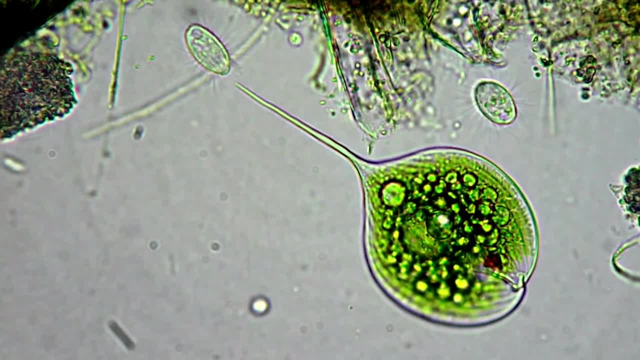 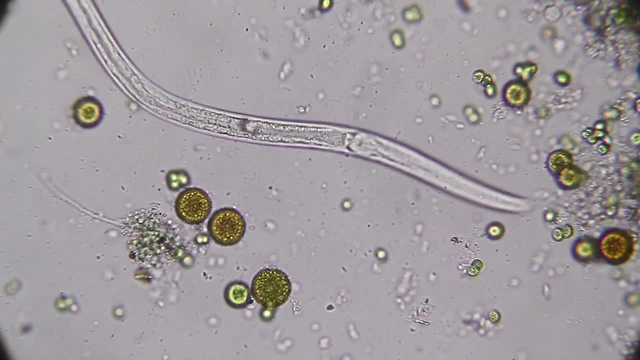 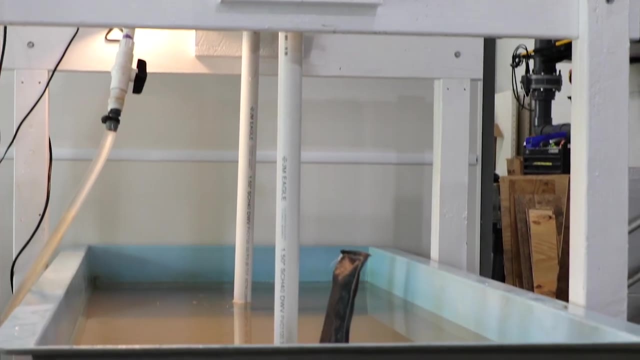 In the coming months, filter-feeding hydrazones, worms, shrimp and crabs will grow alongside them and become threats. Filtering the water as a circulating system keeps predators and silt out, but now an aquaculturist will have to provide clean, nutritious food in high concentration without losing it to. 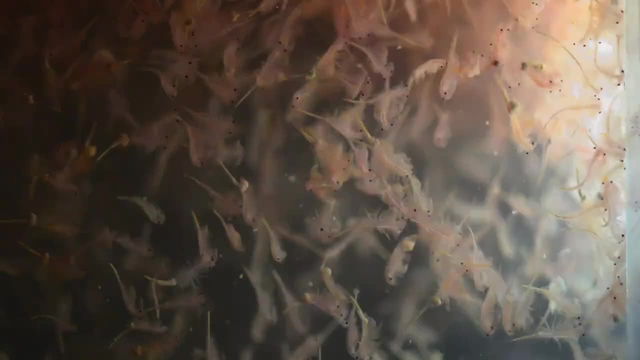 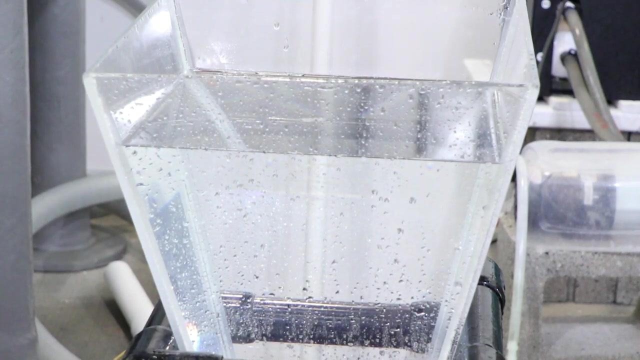 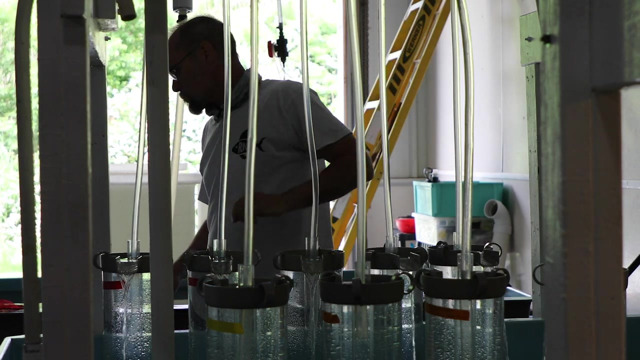 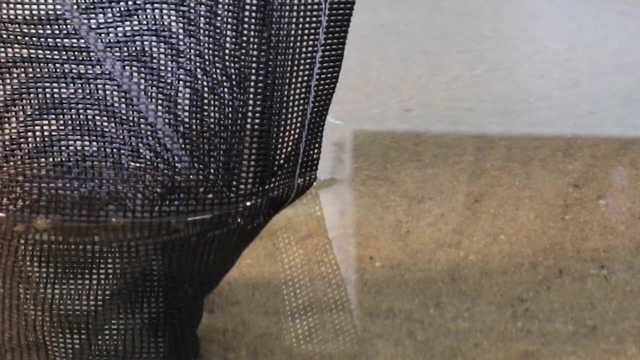 the filter system. That food, mostly brine shrimp, has to be cultured in a parallel aquarium system. Further, not enough is really known about the young crab's nutritional needs to provide a diet as rich as their natural diet. Where are the trade-offs that yield the most survivors for a reasonable cost? At some point the crabs are large enough that their chances in the wild are greatly improved And further effort to care for them is unavoidable. But what is that point? Months One, year Two? Very little is known about survivorship in the wild, because juveniles can move around.